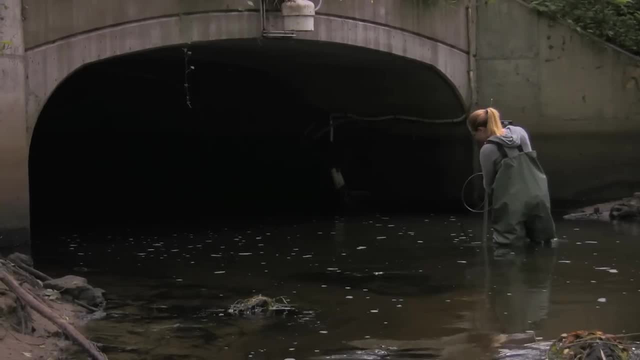 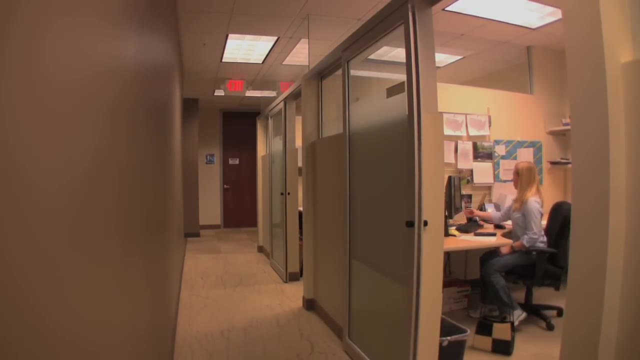 variety that I have in my job. I alternate between working in the field and working in the office, and I think that's a really nice balance. Barr does water quality work around the state of Minnesota and occasionally in other states, so I have traveled to different. 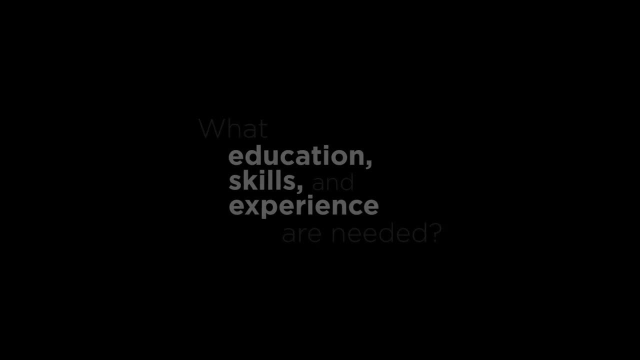 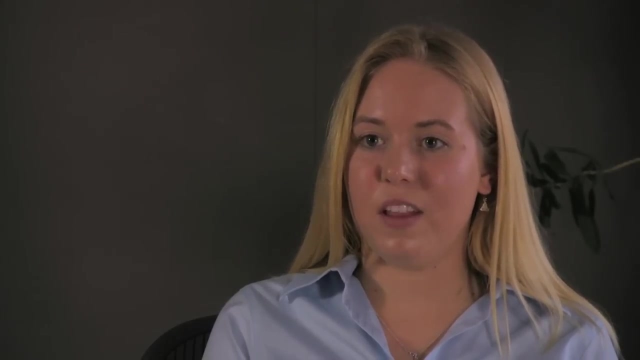 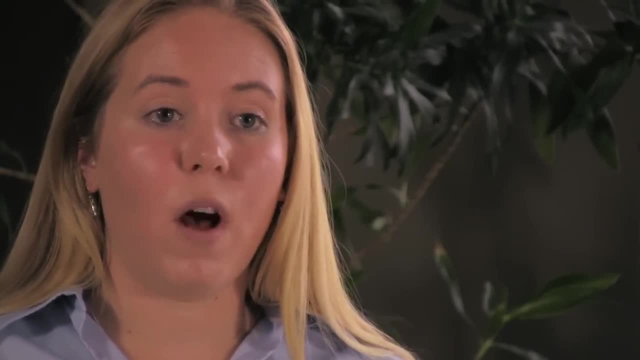 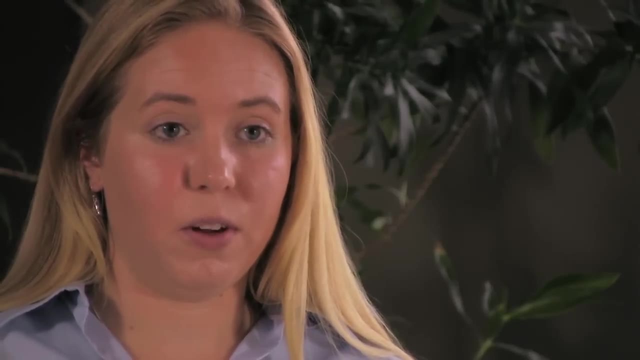 I have a bachelors of science in civil engineering from Marquette University and while I was a student there, I spent two summers as an intern here at Barr And that was a really important experience because it showed me that I liked engineering and it was a good 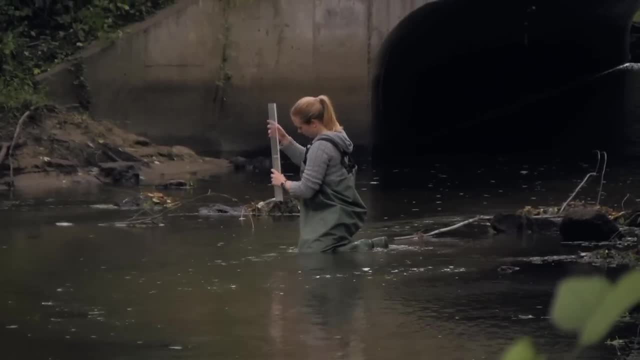 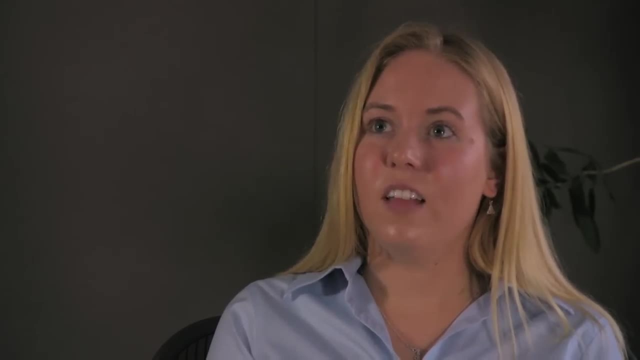 fit for me, And it also showed me that what I was most interested in in civil engineering was water. I looked around and I saw a lot of people with Master's degrees, and so I thought I should probably have one too. After I finished my undergrad, I went straight to graduate school. 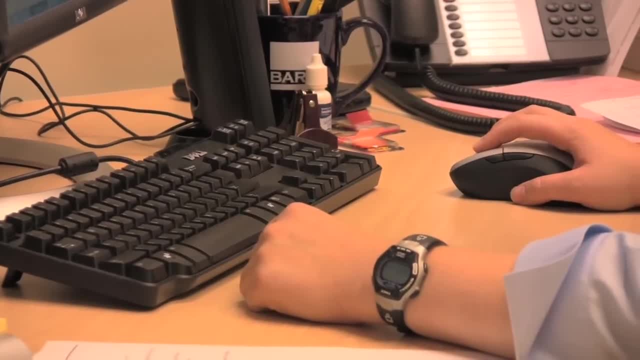 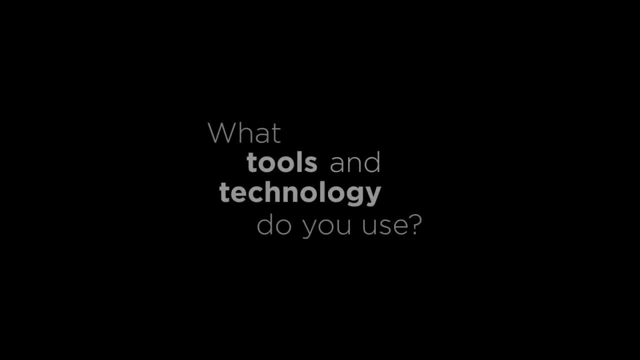 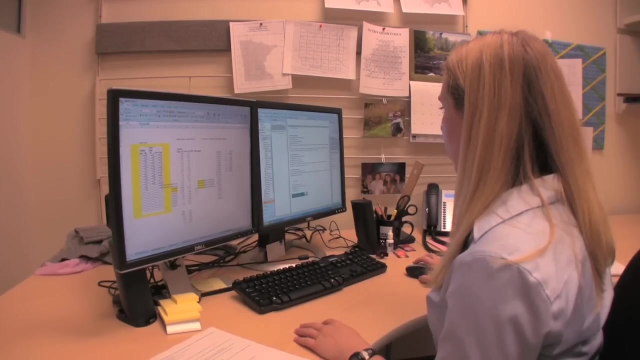 When you're solving problems, it always helps to be a critical thinker and sort of look at the problem broadly and try to come at it from a number of different aspects. Every day at work I use a computer. I use it to keep an eye on the weather. 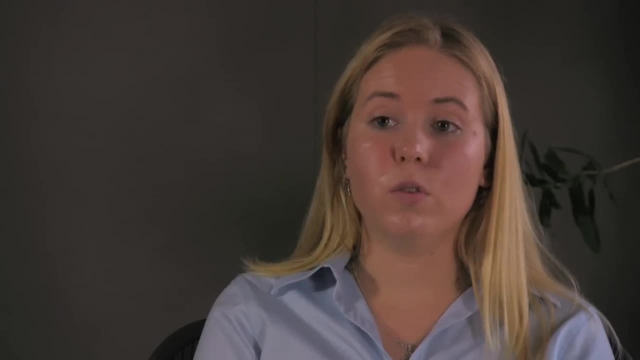 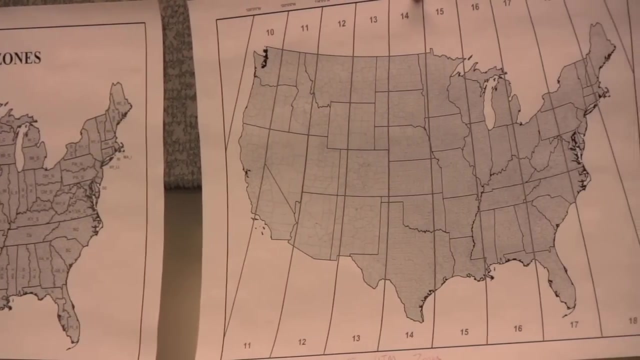 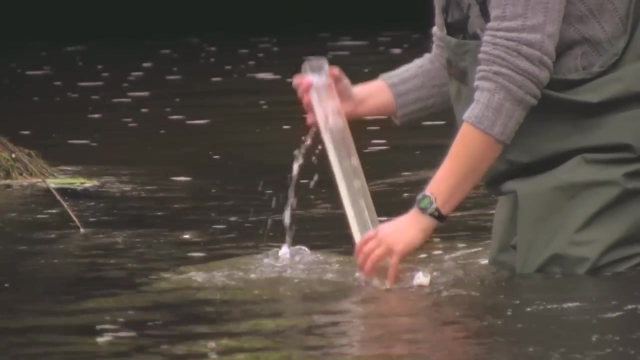 I use it to write up memos and reports. I also use GIS, which is geographic information software. That's been a very valuable skill for me. I use it almost every day. I produce a lot of maps for different projects. When I'm working in the field, I use tools like a transparency tube, which allows me 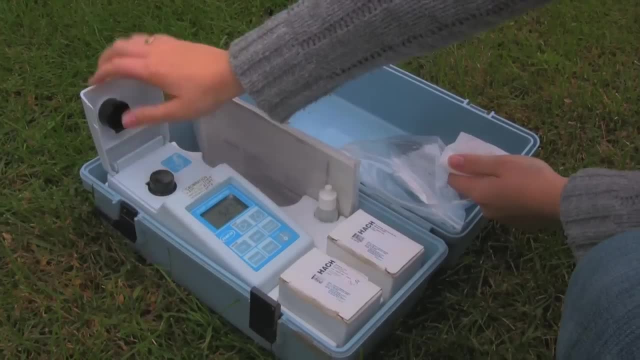 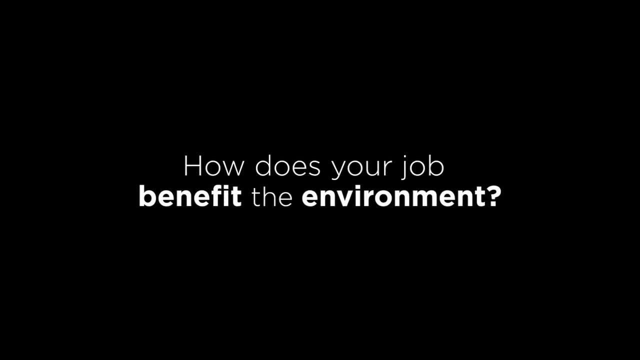 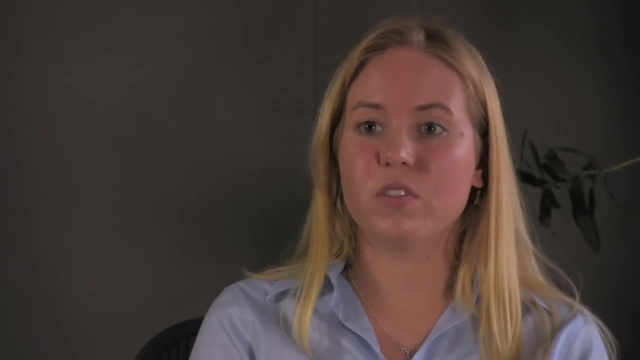 to see how clear the water is. I use a turbidimeter, which is a small machine that uses light, to also measure water clarity. Increased concrete, increased pavement. You know, building a new shopping mall or suburb Subdivision has an effect on the rivers.